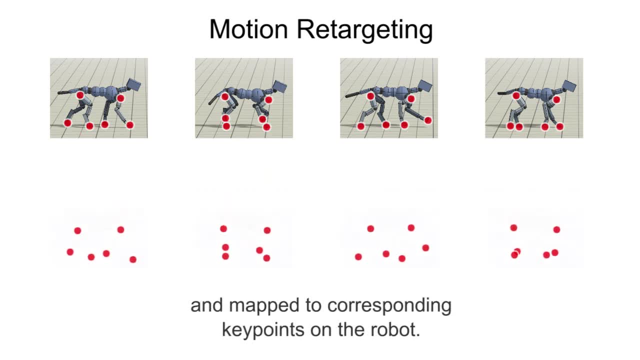 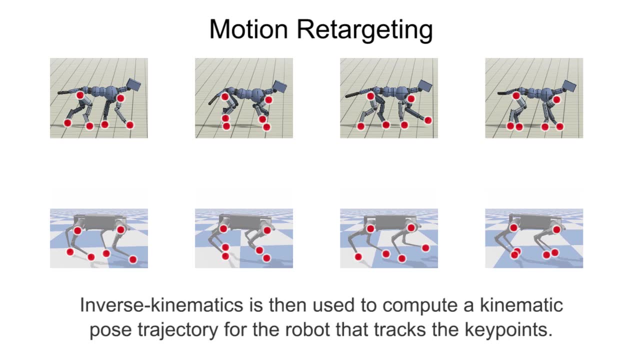 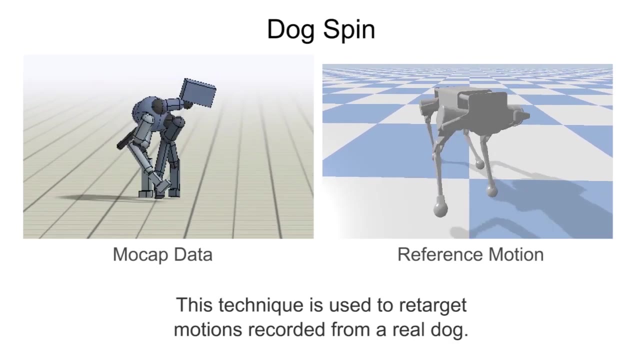 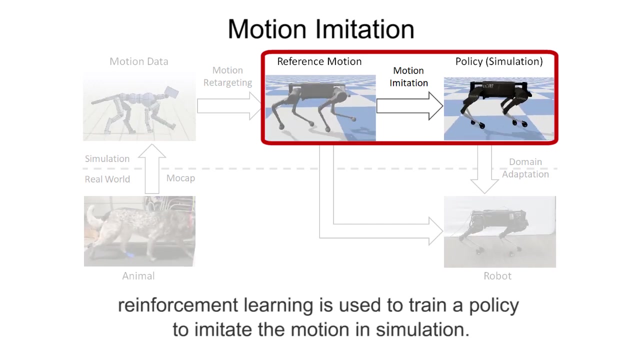 and mapped to corresponding key points on the robot. Inverse kinematics is then used to compute a kinematic pose trajectory for the robot that tracks the key points. This technique is used to retarget motions recorded from a real dog. Once the motion has been retargeted, reinforcement learning is used to train a policy to imitate the 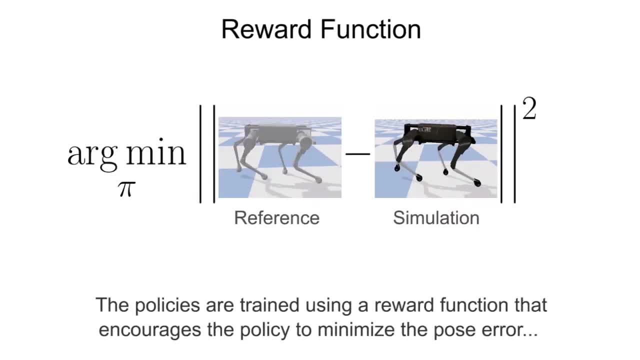 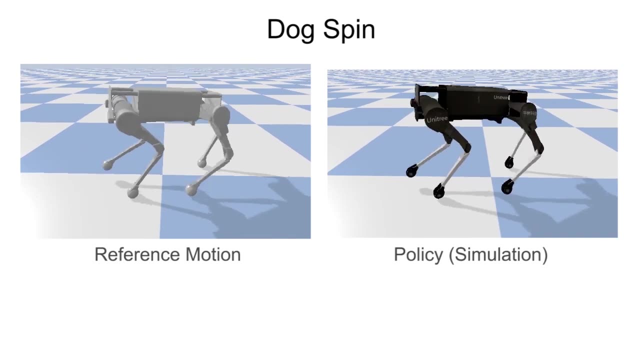 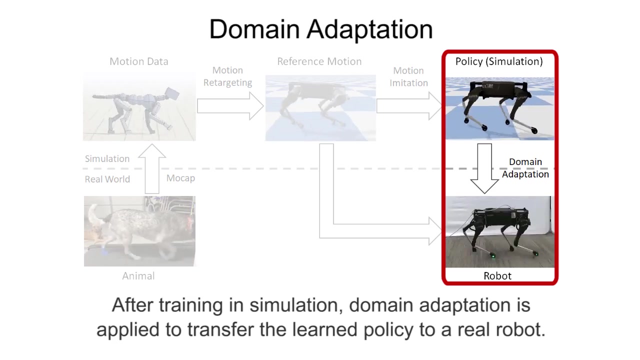 motion in simulation, The policies are trained using a reward function that encourages a policy to minimize the pose error between the reference motion and the simulated robot. The same reward function is used to learn all skills After training in simulation domain. adaptation is applied to transfer the learned policy to a real robot. 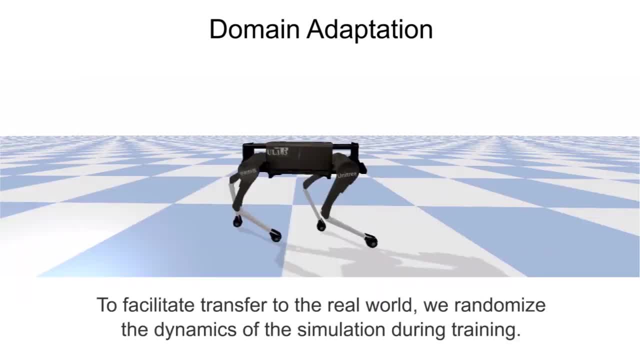 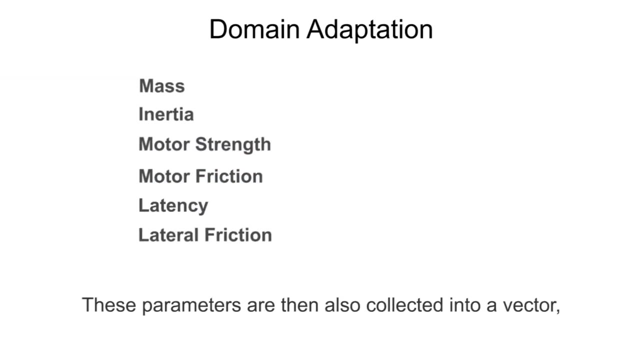 Add nothing. To facilitate transfer to the real world, we randomized the dynamics of the simulation during training. The dynamics parameters include mass inertia, motor strength, motor friction, latency and lateral friction. These parameters are then also collected into a vector and encoded into a latent dynamics representation. 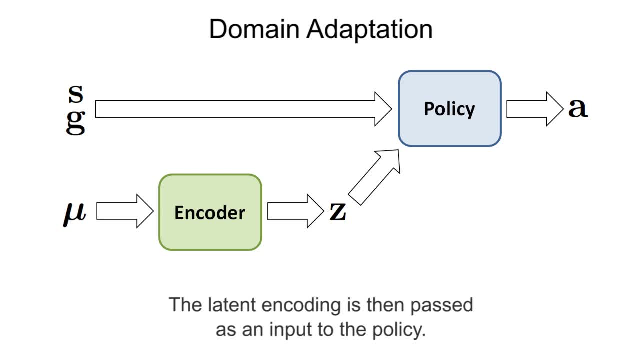 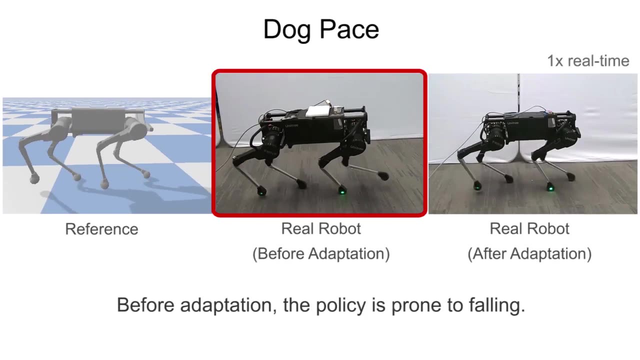 The latent encoding is then passed as an input to the policy. After transferring the policy to the real world, the encoder is removed and we directly search for a latent encoding that enables the policy to execute the skill with the real robot Before adaptation. the policy is prone to falling. 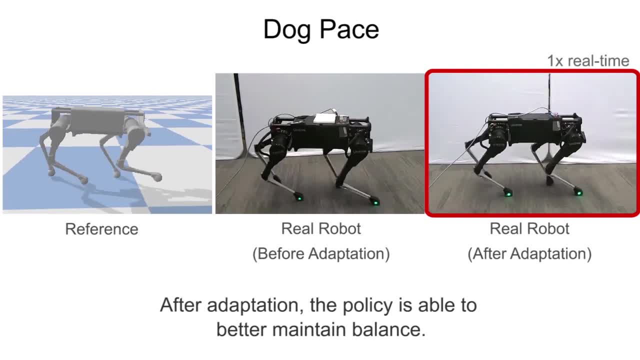 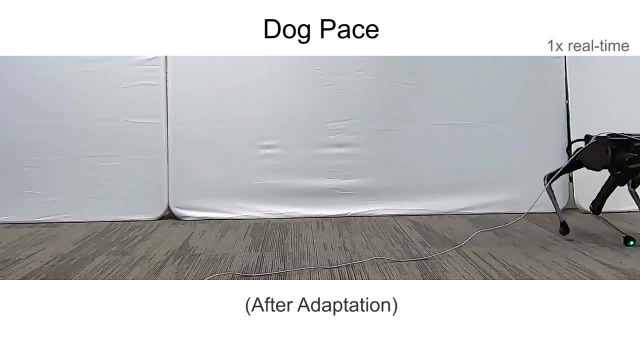 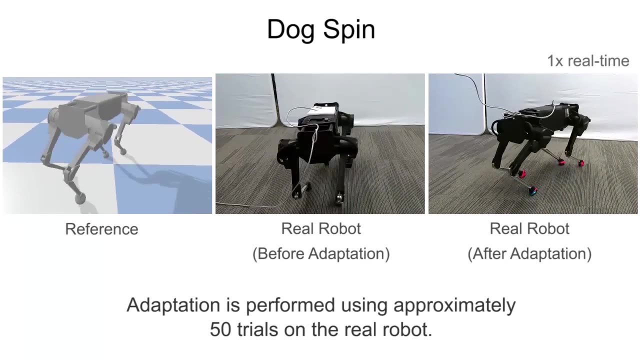 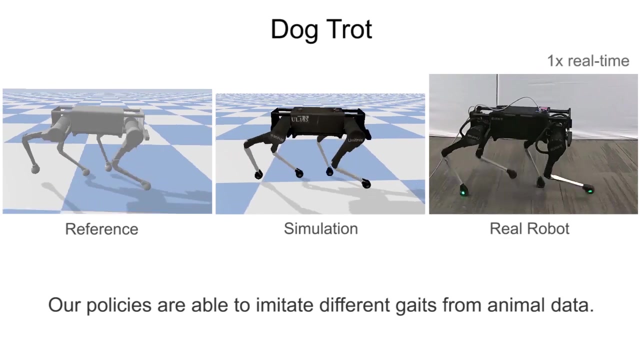 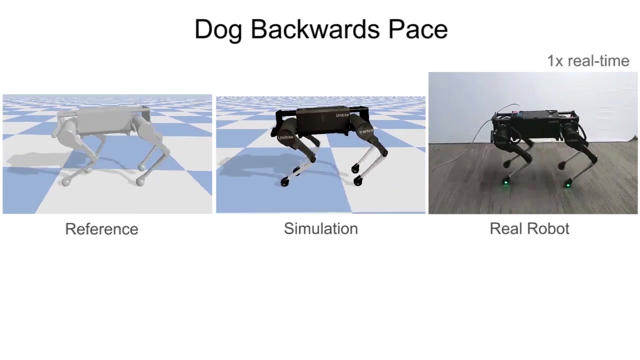 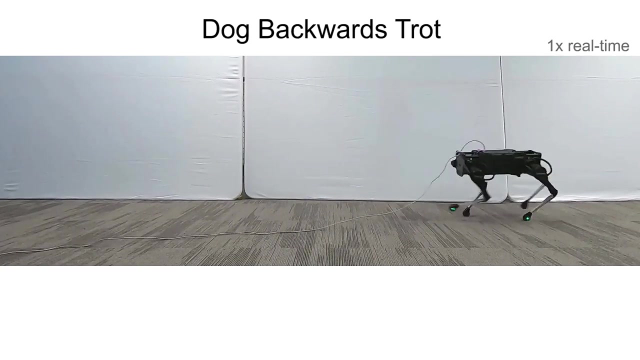 After adaptation, the policy is able to better maintain balance. Adaptation is performed using approximately 50 tries. Our policies are able to imitate different gaits from animal data. Our system can also imitate motions from artist-generated keyframe animations. Our system can also imitate motions from artist-generated keyframe animations. 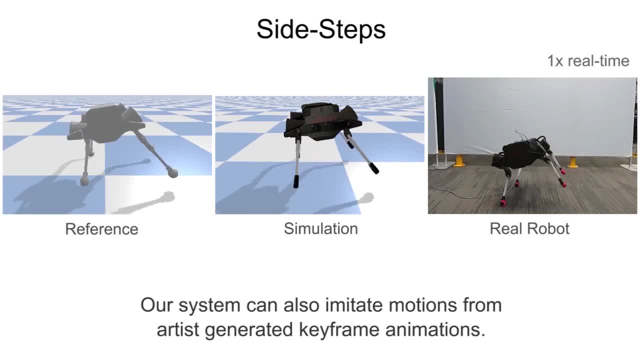 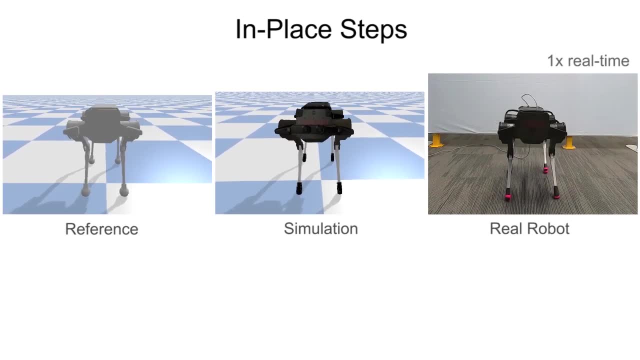 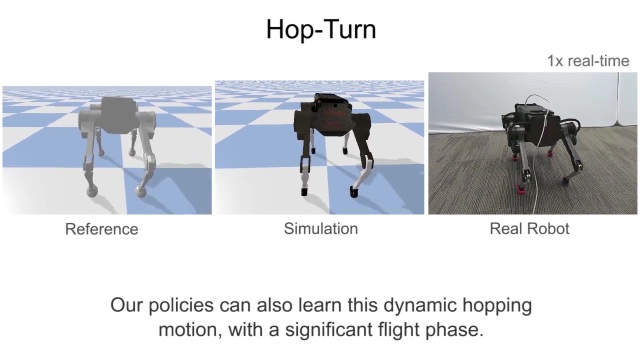 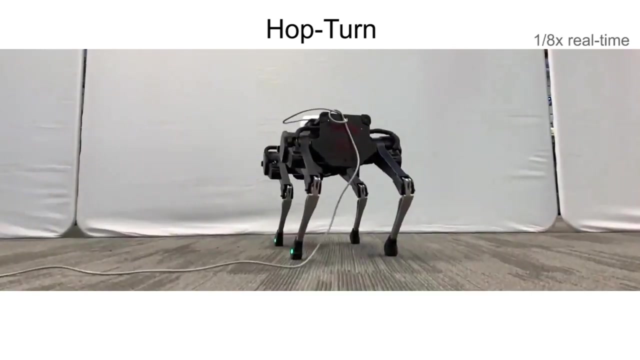 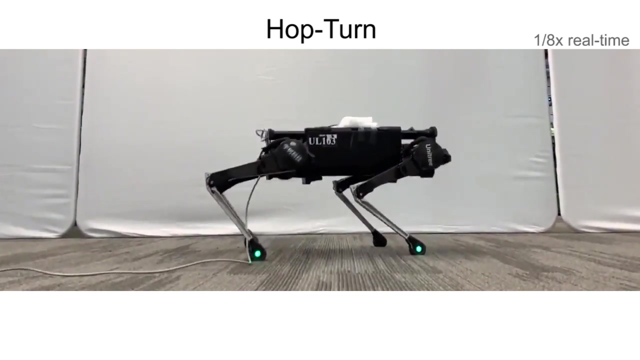 Our system can also imitate motions from artist-generated keyframe animations. Our policies can also learn this dynamic hopping motion with a significant flight phase. Our policies can also learn this dynamic hopping motion with a significant flight phase. Our policies can also learn this dynamic hopping motion with a significant flight phase. 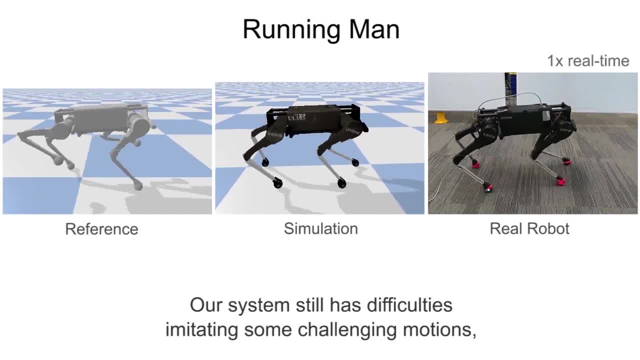 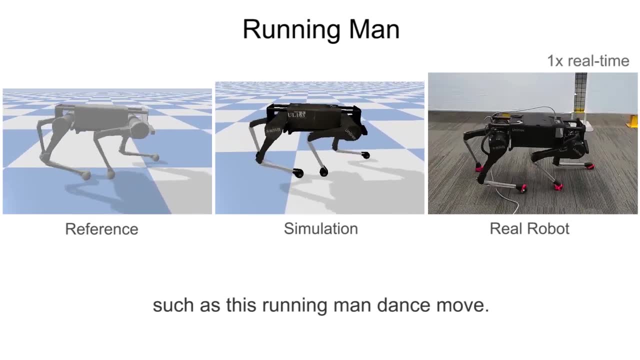 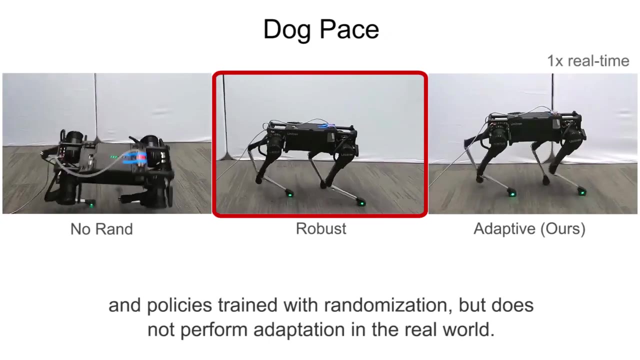 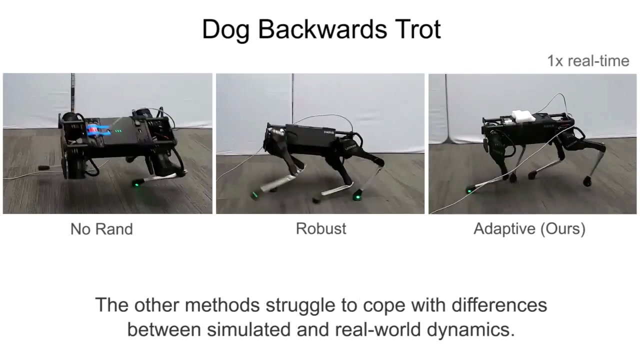 Our system still has difficulties imitating some challenging motions such as this running man dance move. Next, we compare our method to baseline policies trained without domain randomization. in simulation such as this running man dance move Policies trains with randomization but does not perform adaptation in the real world. 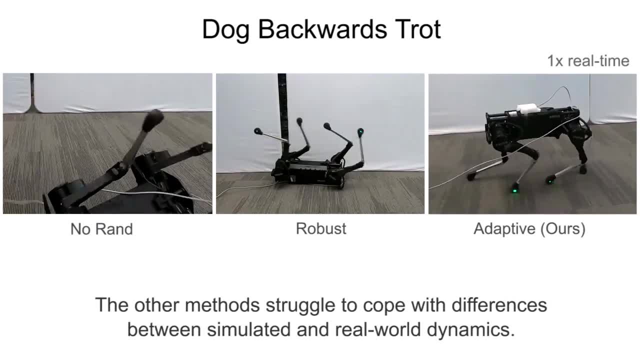 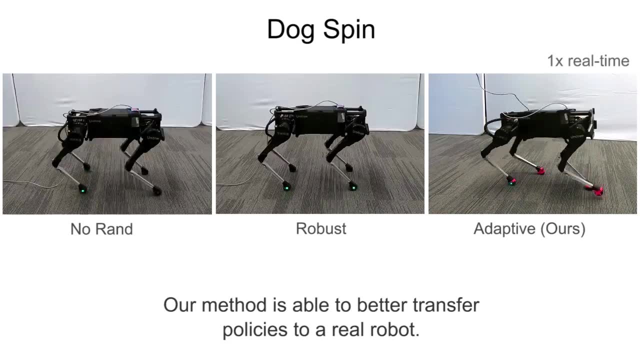 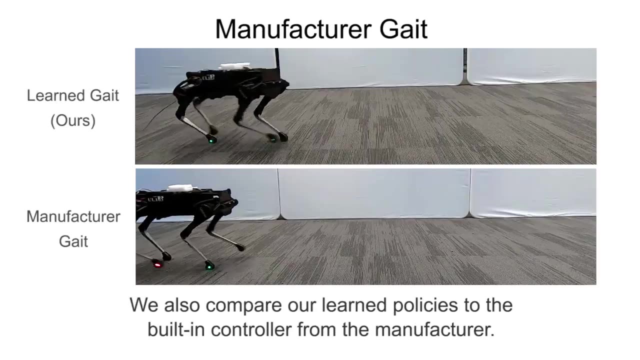 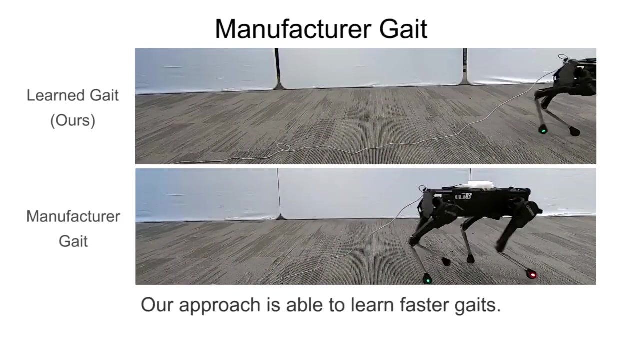 The other methods struggle to cope with differences between simulated and real-world dynamics. Our method is able to better transfer policies to a real robot. We also compare our learned policies to the built-in controller from the manufacturer. Our approach is able to learn faster gates. More details are available in the paper. Thanks for watching.